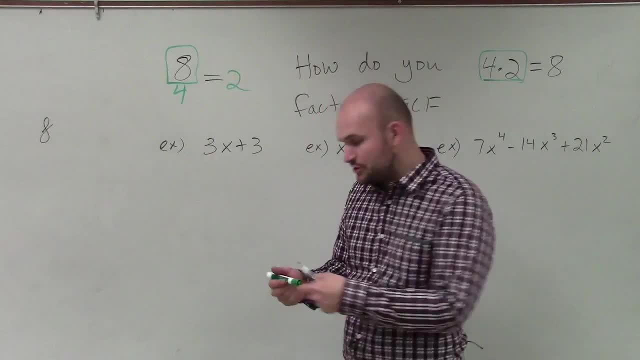 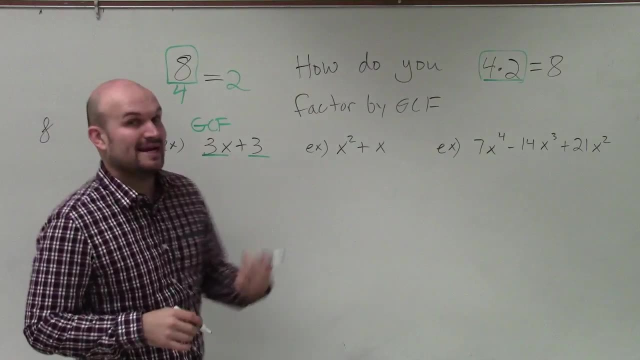 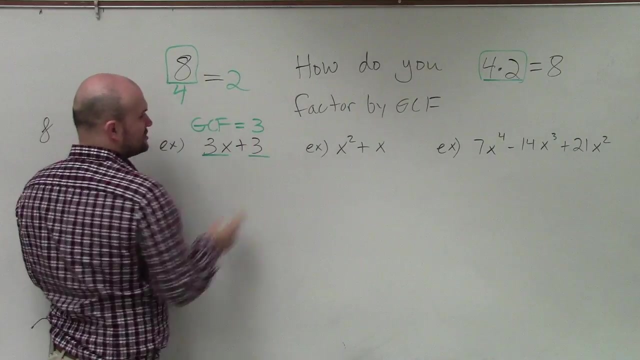 we're going to determine a number or a variable that divides into both of my terms, And what we call that term is our GCF. And the GCF represents greatest common factor, Common factor between both of these. Now you can see that the greatest common factor of this binomial here is just 3.. 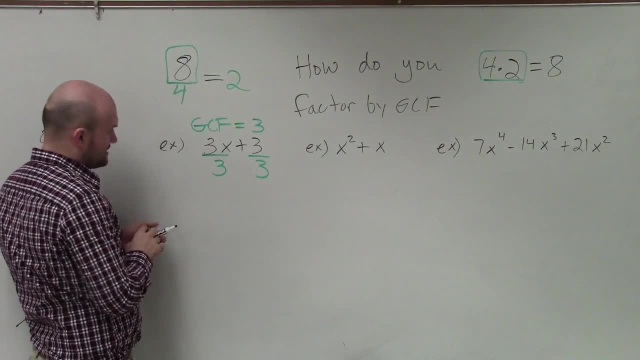 So what I'm going to do is I'm going to divide by 3,, just like I did with the number 8.. Then, since I'm dividing by 3, I'm going to rewrite that as the product times its quotient. Well, 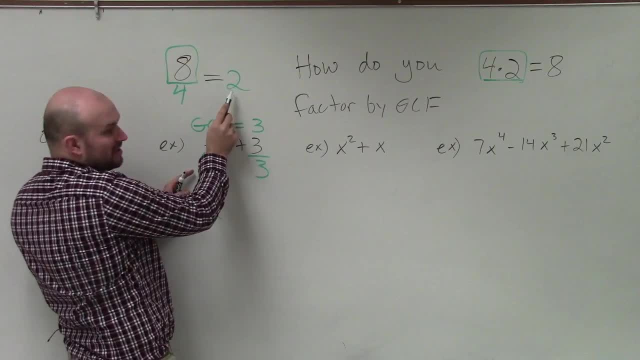 the quotient is the number 8.. So I'm going to divide by 3, just like I did with the number 8.. So the quotient of this divided by 3 is not just going to be a single number, like it was 2. It's. 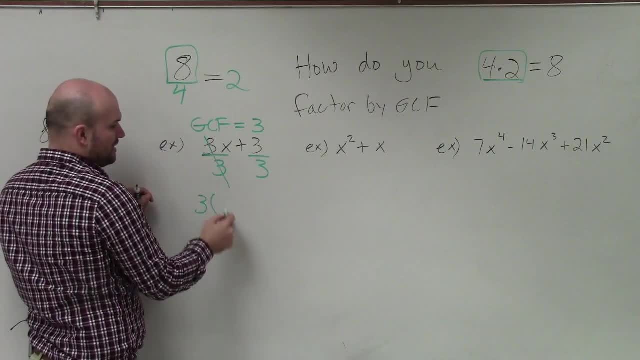 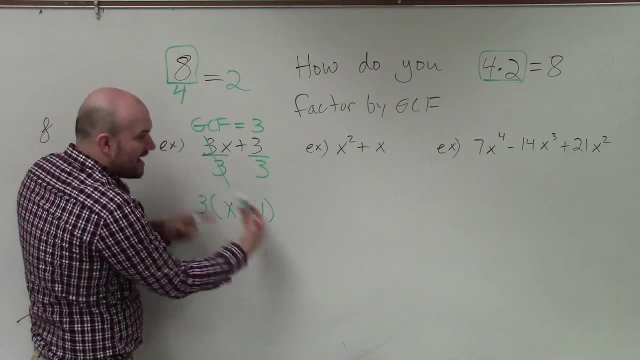 going to be an expression: 3x divided by 3.. Those go to 1.. It's just going to be x, 3 divided by 3 is positive 1.. Now I have factored out the GCF. See the GCF is 3.. I have divided it out. 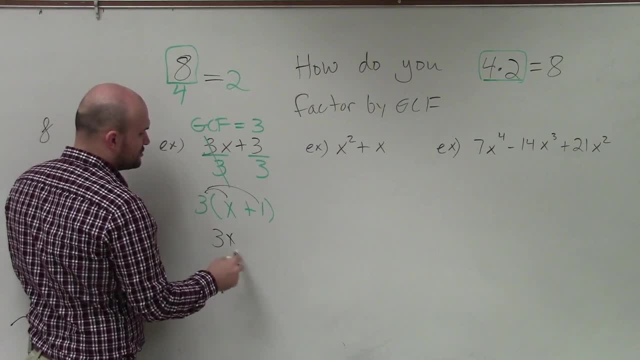 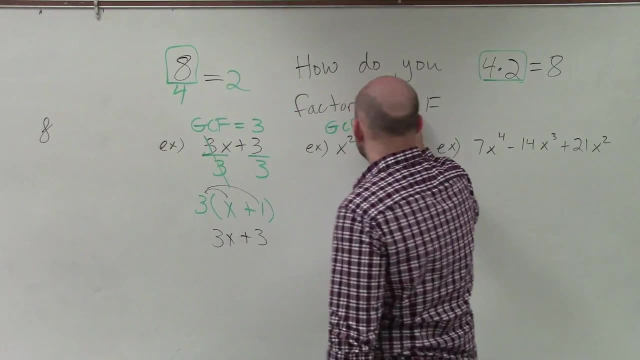 And we can always check our answer by applying the distributive property. For here you can determine that the GCF is not a number. But now the GCF is going to be a variable, which is x. So I'm going to divide by x and both of them. So I'm going to divide by x and 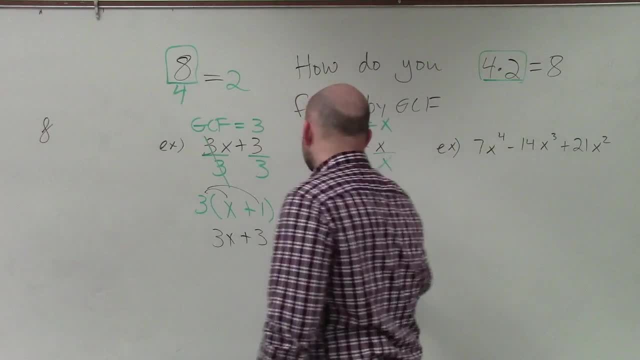 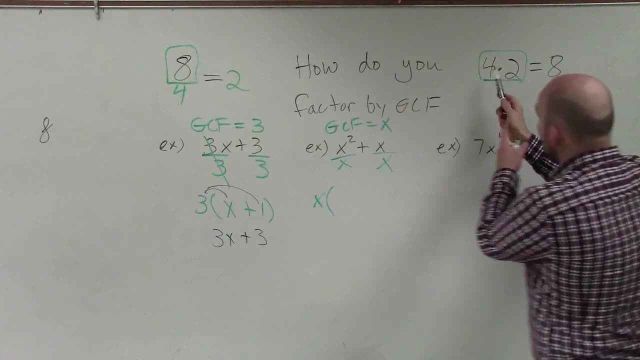 both of them. And again, once I take my variable x, I factor it on the outside And then I multiply it by our quotient. So I divide it and then multiply my divisor by the quotient Divisor by quotient x squared divided by x. here, using the properties of exponents, I'm just left with 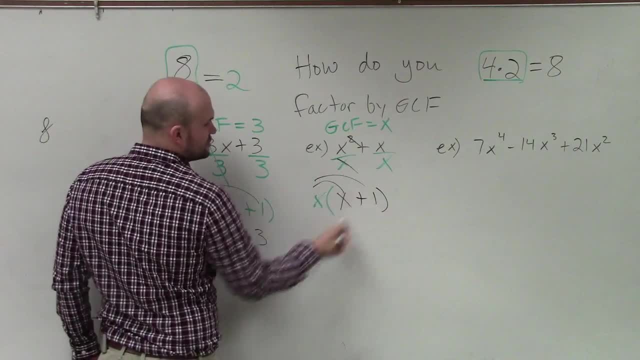 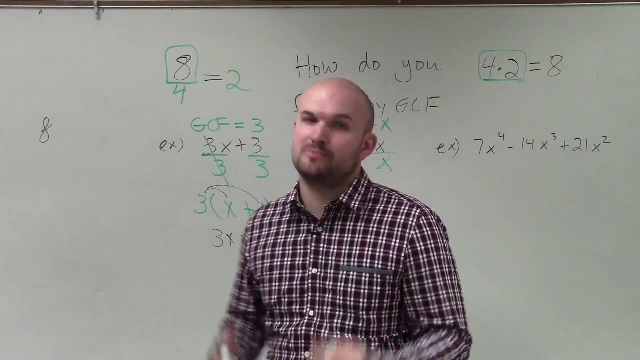 x. x divided by x is positive 1.. Again, check my answer: x squared plus x. Now, lastly, this is not limited to just binomials. We could also divide trinomials or polynomials with 4,, 5,, 6. 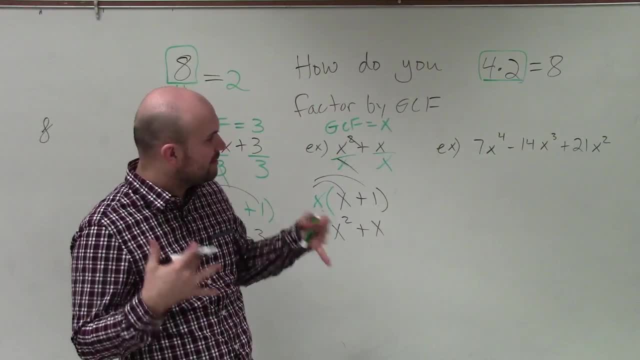 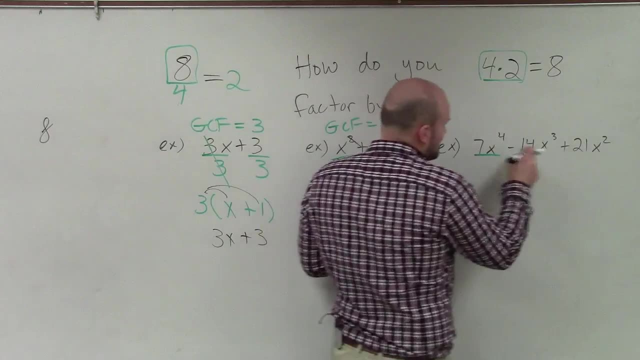 terms. So in this one it gets a little bit more confusing because we want again to identify what is the largest number and variable that divides evenly into all three of these terms. All three of these are separate terms, separate monomials that we need to divide into. So in our case, 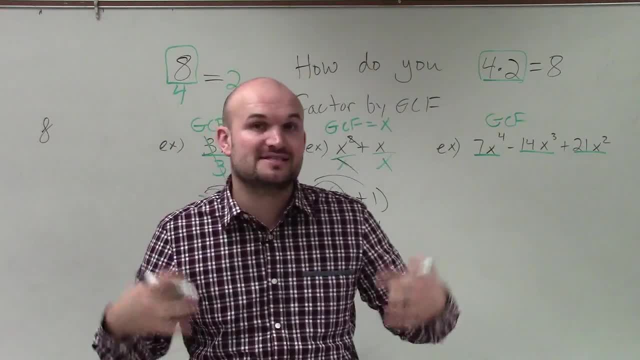 the GCF. if you're looking for the largest number that divides into all of them, you want to kind of look at the smallest of terms. Well, the smallest number here is 7.. Does 7 divide into 7,, 14, and? 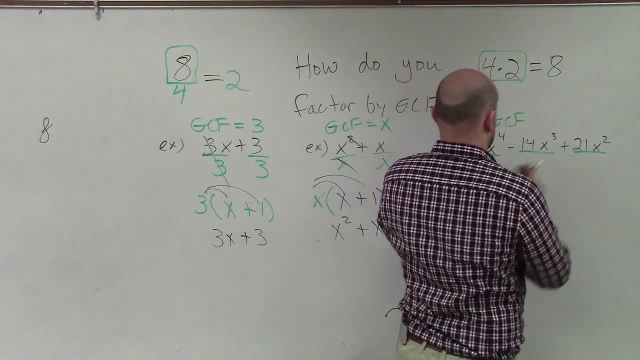 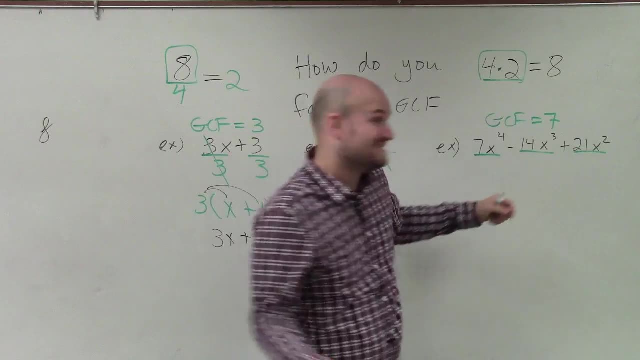 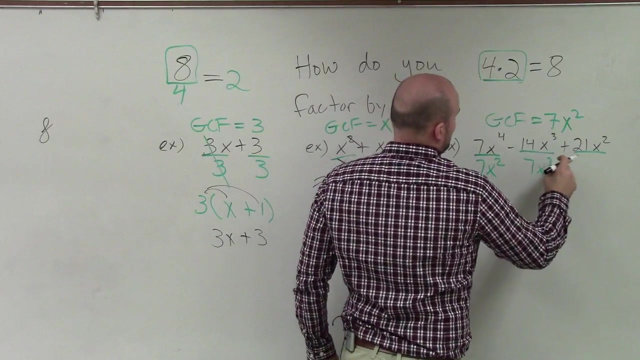 21?? Yes, And that is the largest number that's going to do that. Then we look at the variables. Well, the smallest variable is x squared. Does x squared divide into x cubed x fourth? Yes, it does So. I divide every single term by 7x squared, because that is the 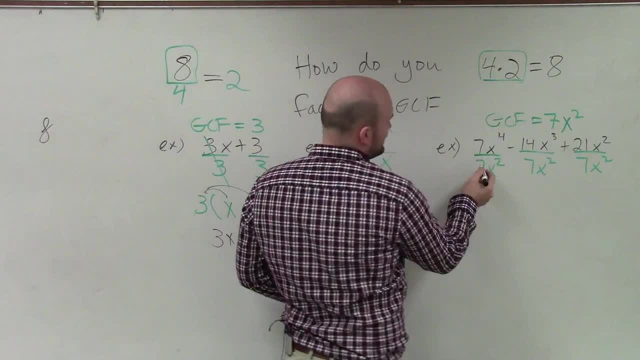 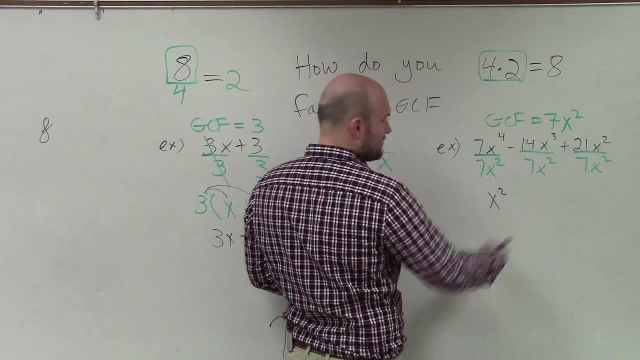 largest term that can evenly divide into each term. Here I have 7 divided by 7, which is just 1.. x to the fourth divided by x squared. Remember you subtract the exponent, so that's just x squared. Here I have negative 14 divided by 2, which is a quarter. So I have 7 divided by 7,. 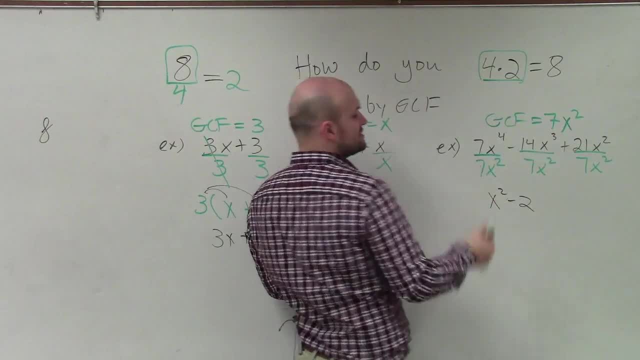 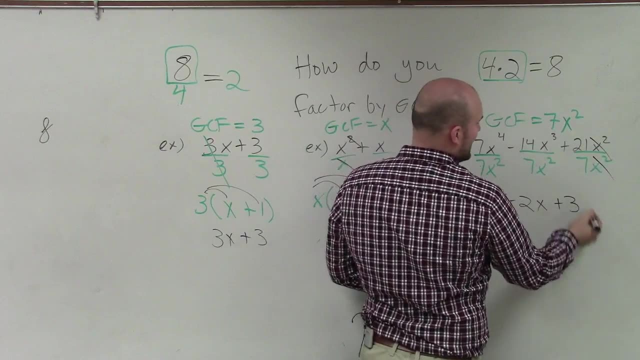 which is a negative 2.. x cubed minus x squared is x3 minus 2, which is just x to the first power. And here I have 21 divided by 7, which is a positive 3.. And then the x squareds divide out. 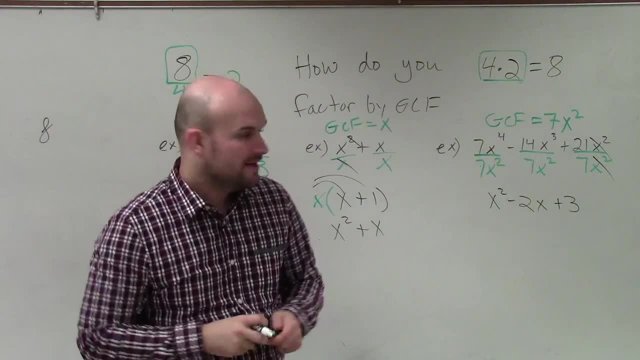 to 1.. So I'm just left with x squared minus 2x plus 3.. So there you go, ladies and gentlemen. That is how you factor out the GCF from a polynomial. Thanks. 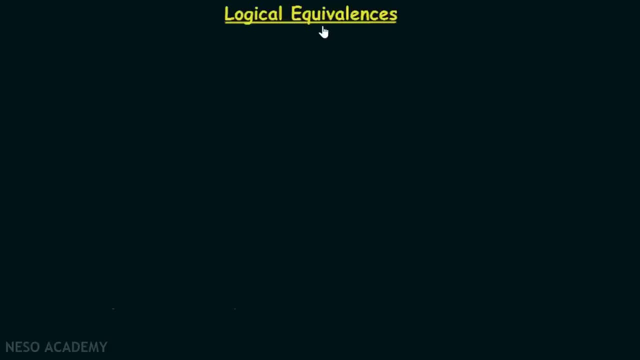 In this lecture we are going to talk about the logical equivalences. 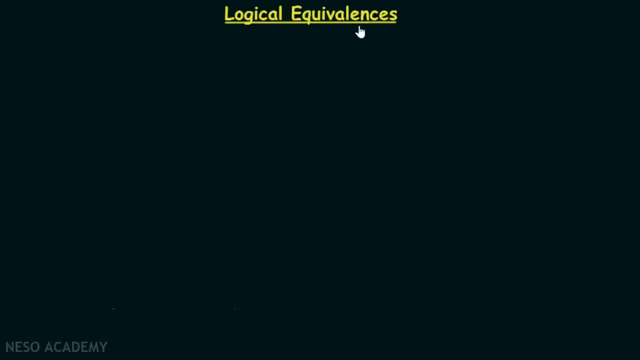 Now let's consider the definition of logical equivalence. 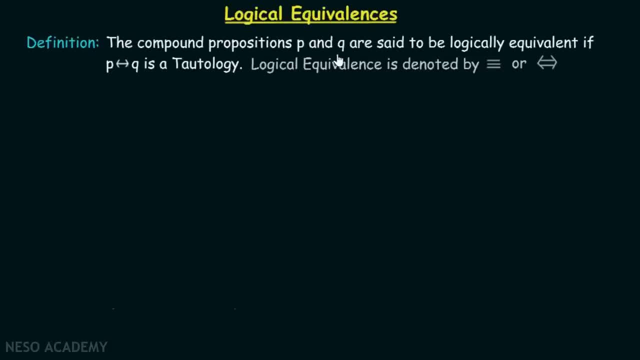 The compound propositions P and Q are said to be logically equivalent if P bi-conditional operator Q is a tautology. 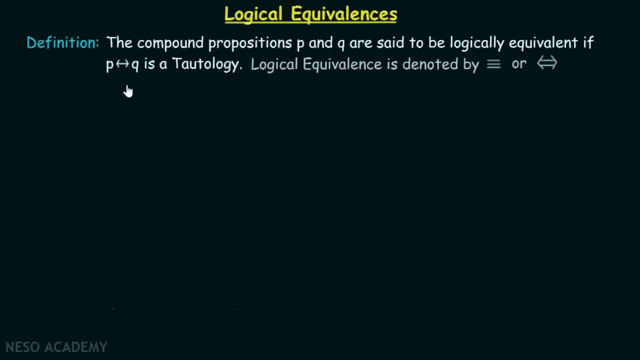 Now what does it really mean? When P is true, then Q has to be true and when P is false, then Q has to be false. 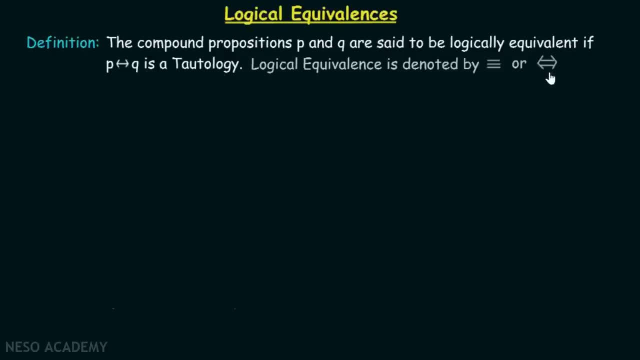 Logical equivalence is denoted by this sign or this sign. Let's consider one example. 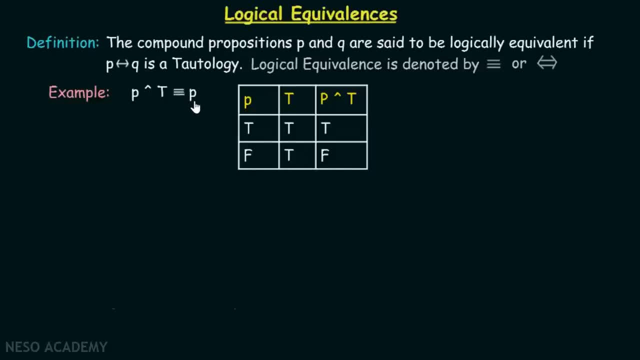 P and true is equivalent to P. How we can say that P and true is equivalent to P? 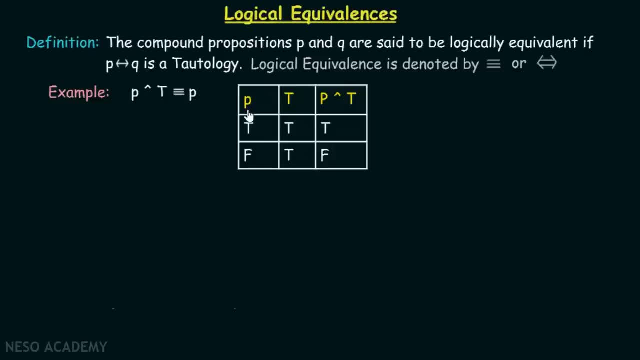 Let's try to understand with the help of the truth table. Let P be the proposition. There are two possible truth values for this proposition that is true or false.